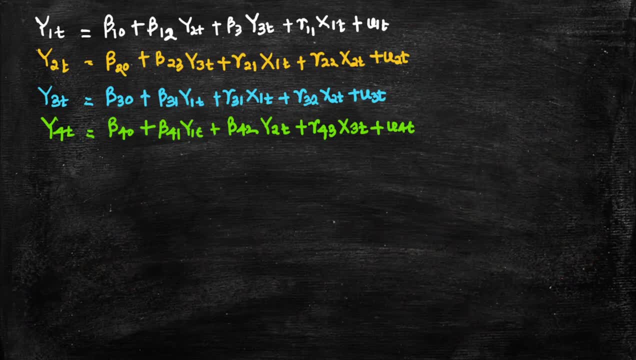 thing to do is arrange these equations into very friendly matrix format. Okay, So we are going to do this in such a way that we can form the matrix afterward. Okay, In order to do that, what we do is: you take the right side of the equation, these things, okay. 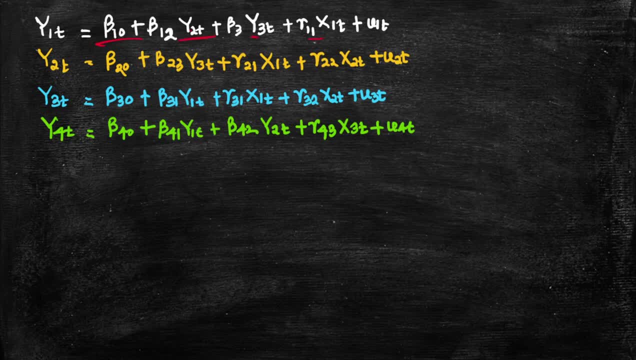 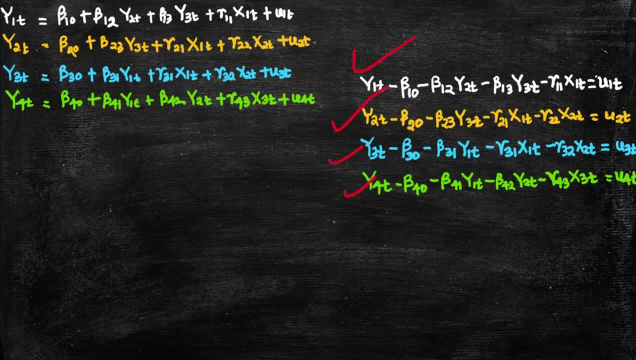 to the left side. Okay, So you will get like some equation like this: Okay, Like this you will get. Okay- Sometimes in some books also, you can find it In a different way- where you will get them equal to zero. Okay, You will make them equal. 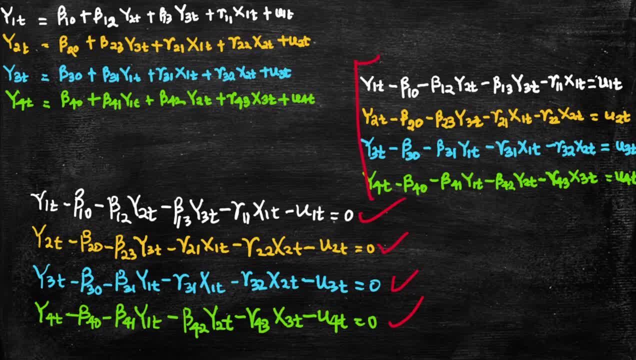 to zero. This is also correct. This is also correct. Either way you can use. Okay, What matters is the matrix. Now, the matrix will be formed from the coefficients of the variables here. Okay, The coefficients of the variables will be. 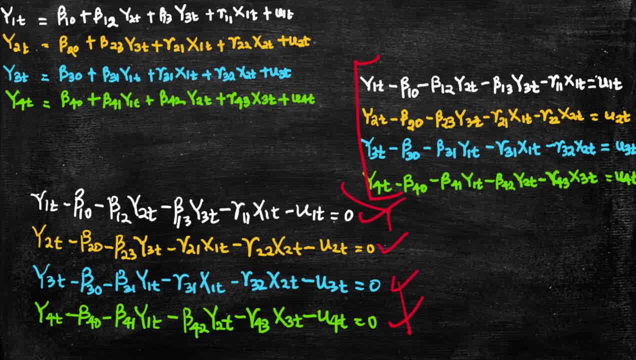 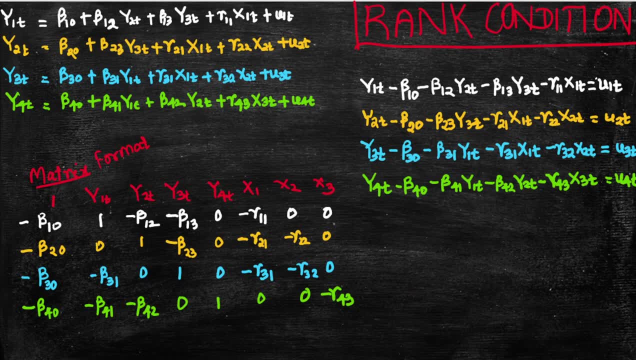 arranged in a matrix format. Now in the next slide we see that the matrix format we have been doing, what you are doing, is you are taking all the variables of the equations- Okay, All the variables in the equations- and putting them in the first row here, Okay, So, 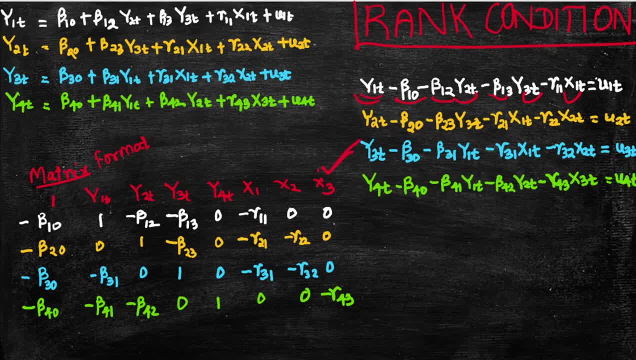 the first row is this one: We are giving the variables. We are keeping the variables Y1t, Y2t, Y3t, Y4t, X1,, X2.. All these are variables, right? So Y1,, Y2,, Y3t, Y4 or Y4t, All these. 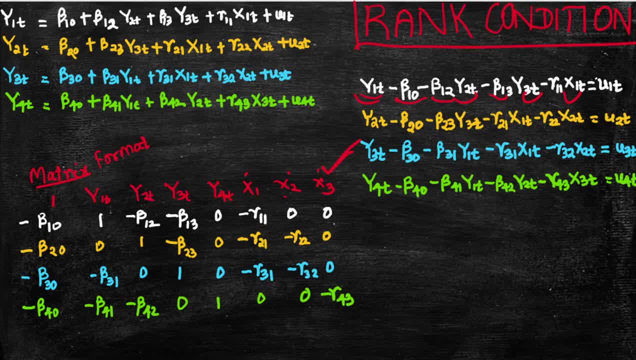 are your endogenous variable and predetermined variable, Three in number: X1, X2, X3.. Okay, Now what you have done is how many times beta 1, here we are keeping this 1 for the intercept. Now beta 10, negative beta 10, here it is coming, negative beta. 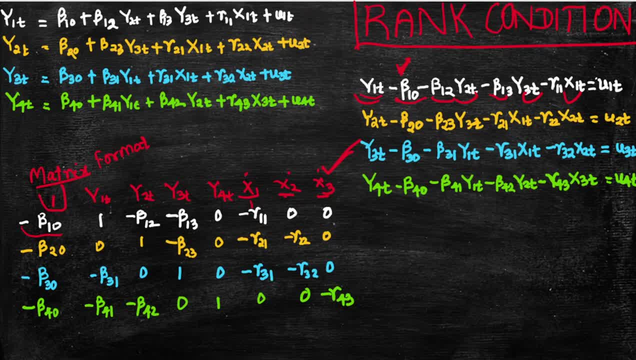 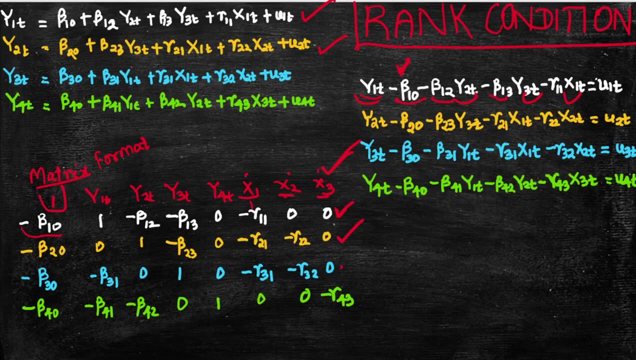 10. This is for the first equation. Now I have highlighted this in the color respective color. So white color coefficients. white color coefficients are for the first equation. Yellow color is for the second equation here, Okay. Blue color for the third one And the 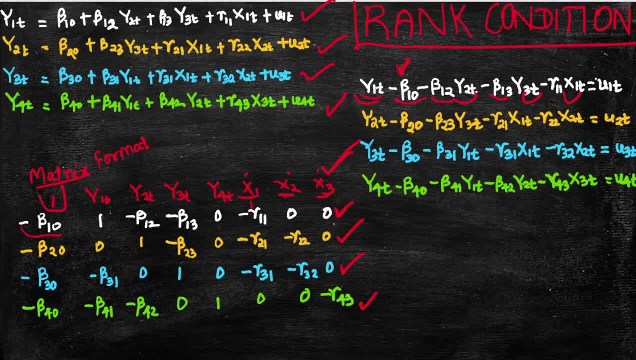 green one. this is the fourth equation: coefficients. Okay, No confusion. Now these are the coefficients associated with that, variables in that particular equation. So if you are talking about third equation, so this is our third equation, Number 3, and we have changed that to this one. Okay, From here we can see that Y3t is. 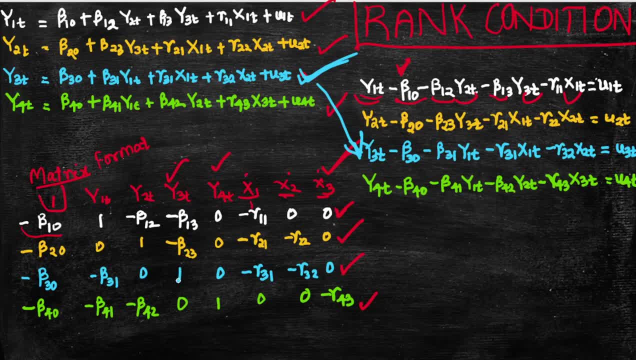 present. so whatever Y3t is there for third equation, we are writing 1 here. Okay. Then next is beta 30. Beta 30 is the intercept. We have written it already here under the 1.. Okay. Next is beta 30, negative, beta 31,. that is for Y1t. 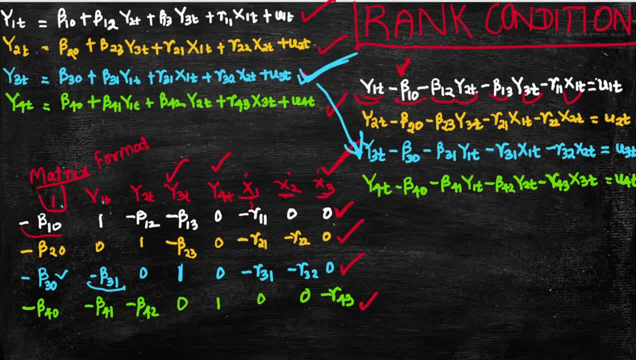 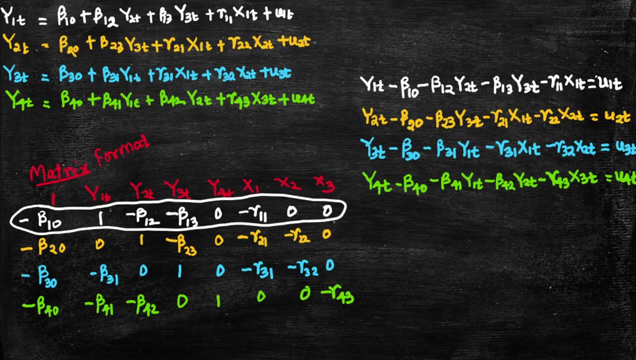 we are writing the respective coefficient associated with that. similarly, for x1 t, we are writing the coefficient that is negative gamma 31. okay, so the sign along with the coefficient. we are writing this coefficient along with the sign here. okay, in the next, what we are going to do is: let's take the equation number one. okay, let's find out whether 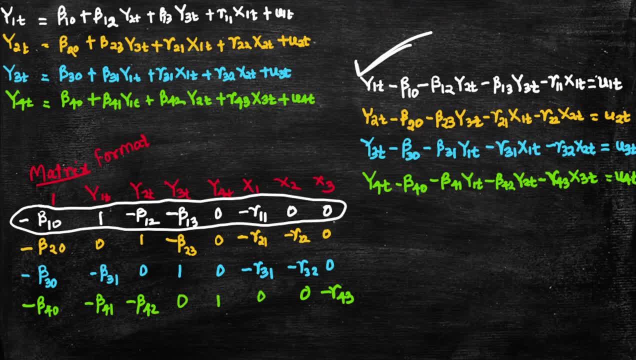 equation one is identified or not. okay, what are the condition? the condition one was: we'll be able to get matrix of the order m minus one. so what is your m here, your capital m here? that is the number of equation, that is four. okay, so we are telling if you could find a matrix using the 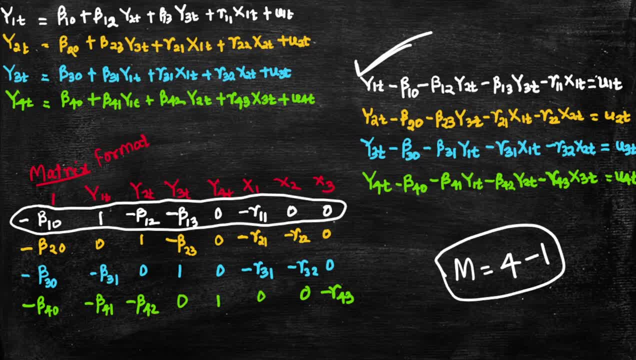 variables. that is excluded from the equation one, then that will be. and that matrix has the determinant of not equal to zero, then we say that it is identified. if the determinant of that matrix is zero, that means the rank of that matrix is less than three. in that case it will be not identified, okay. but if it is not equal to zero, 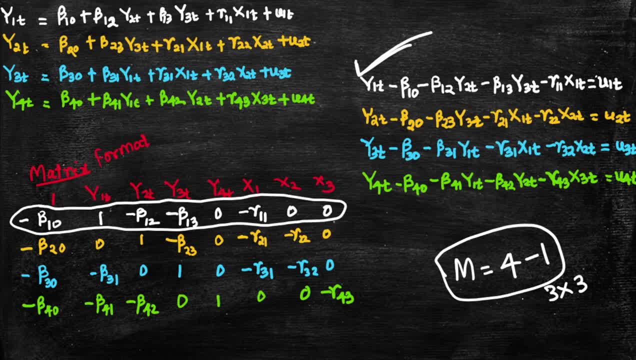 then it is identified. it is going to be identified, we'll see in this case. so, for the equation one, what you have to do is round a circle around the coefficient for equation one, because that row we are not going to consider and what we are going to do is we are going to write the coefficient. 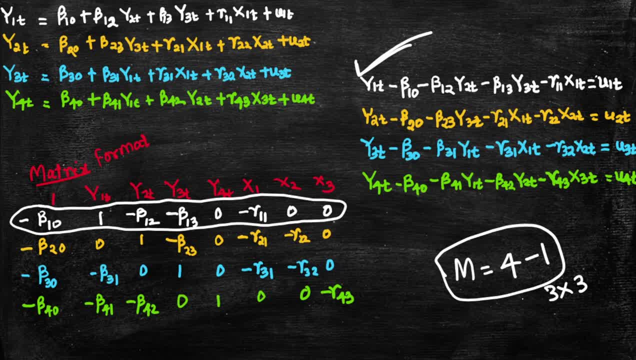 we are going to consider. we are going to consider the variables which were not present in that particular equation. that is, equation number one. so we can see the columns where zero is there. okay, because that variable is not present in the equation. okay, now you got it, so from here we'll 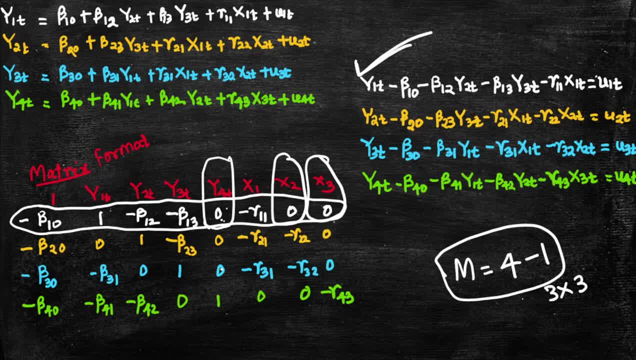 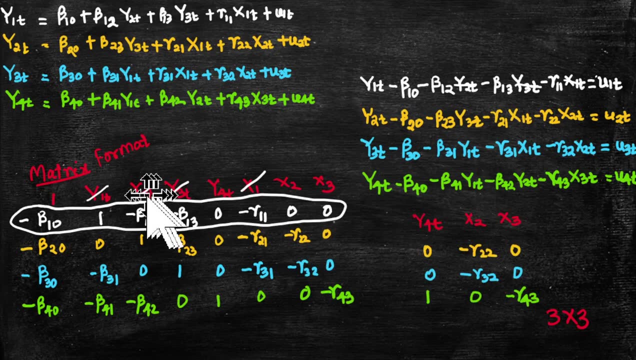 be constructing the matrix. okay, so now you can see here. okay, so you can see that we are canceling out y1d, y2d, y3d, Y4, sorry, y3d then x1. okay, we have strike them out, so we are not going to consider them. 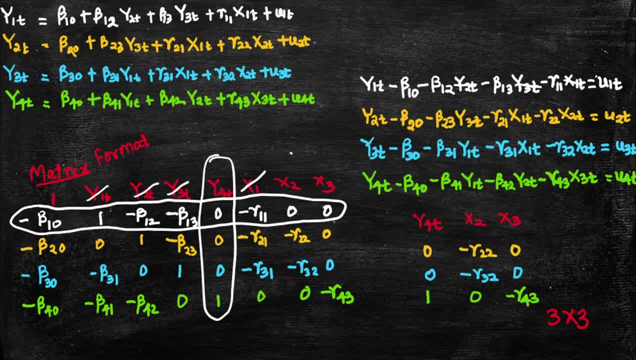 we're only considering the excluded variables, so so from that equation, these are not present in that equation. so we will be considering these values and we are going to ignore these intersection points. okay, so these values will not be there. we are just referring that to find out the values for the matrix. now we are having 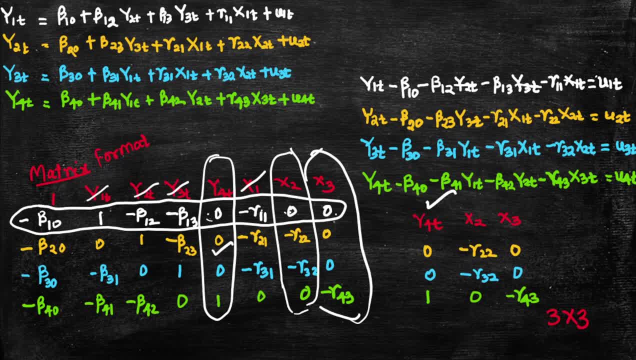 this y 40. for this it is 0, 0, 1 for in the other equation. so you can see that y 40 is not present in equation 1 but it is present in equation 4. right y 40, this one now x 2, is present in. x 2 is present in equation number. 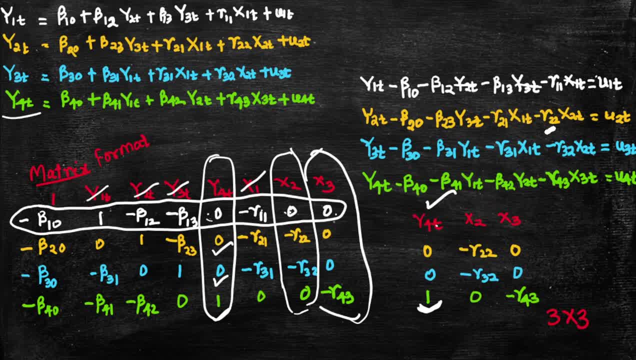 in equation number 2: okay, x 2 t or x 2. i have written x 2 t, okay. okay, fine, you can write it here: t x 3 t, 30. okay, now x 2 t is already present there here, so we're writing negative gamma 2: 2. similarly, in equation 3 is also there x 2 t is there. 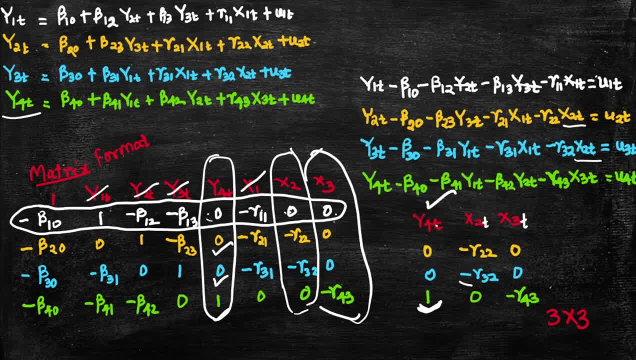 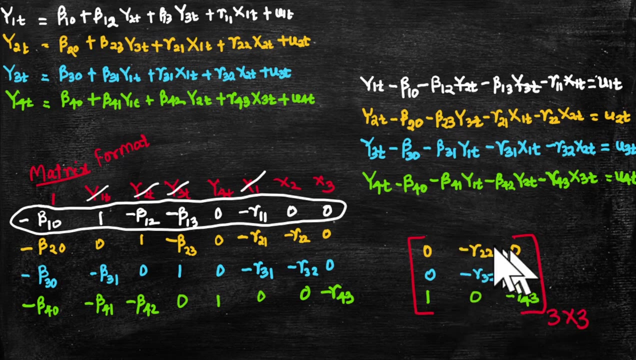 so we are writing the respective coefficient negative, gamma 3, 2 or gamma 32. then for x, 3, t, that is not present in equation 2 or 3, but it is present in equation number 4. okay, then the next thing you have to consider that it is a 3 by 3 matrix, but what about its rank? 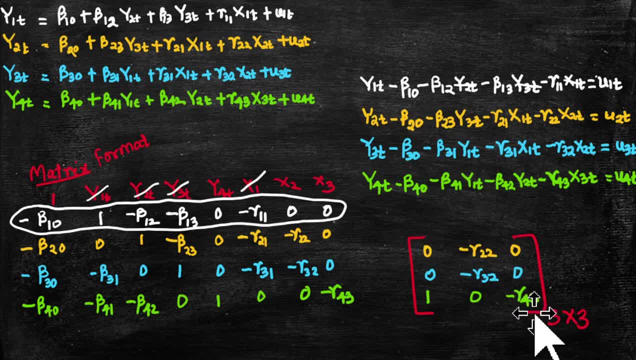 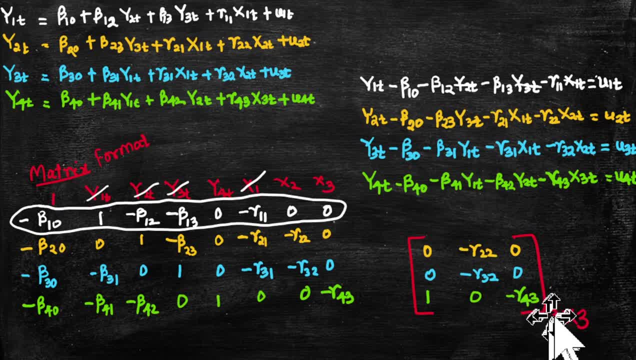 if the rank, if the determinant is not equal, if the rank, if the determinant is not equal to 0, then the, then the rank will be 3 here to 0, then the, then the rank will be 3 here to 0, then the, then the rank will be 3 here. let's see if. what about the determinant? 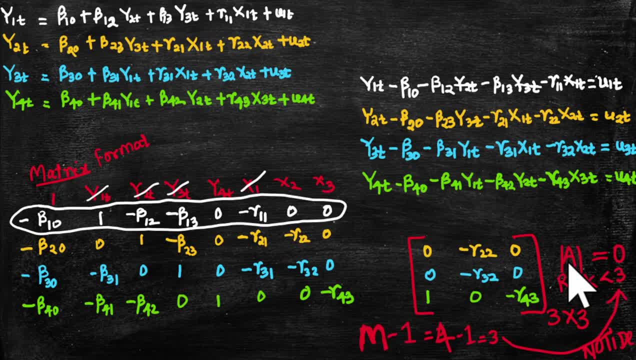 let's see if. what about the determinant? let's see if, what about the determinant value? you can see that, that the value, you can see that, that the value, you can see that, that the determinant of this matrix will be equal. determinant of this matrix will be equal. 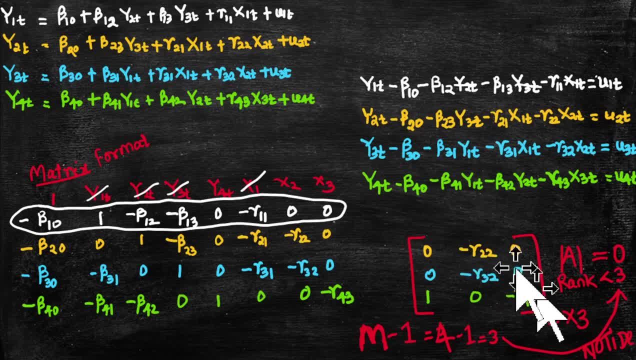 determinant of this matrix will be equal to 0, because it will be multiplied by 0 to 0, because it will be multiplied by 0 to 0, because it will be multiplied by 0 here. okay. so if you do that, then you will here. okay, so if you do that, then you will.